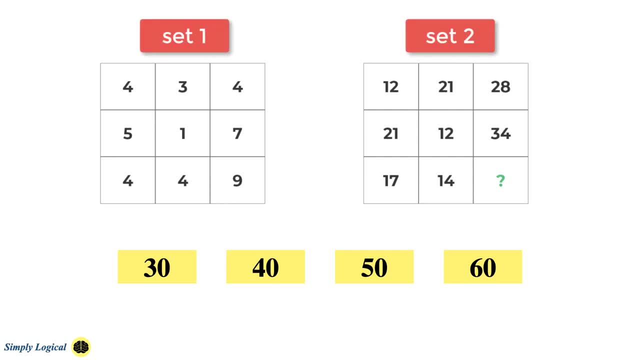 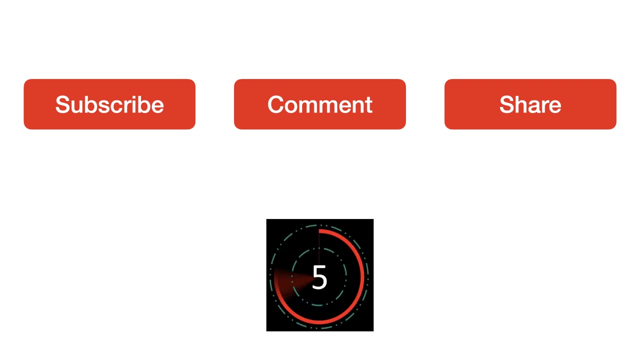 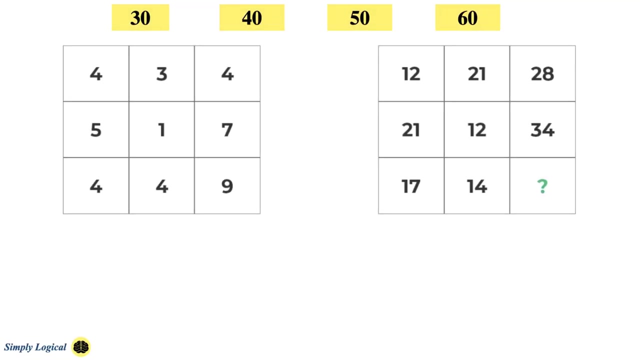 There are 4 options to this particular problem. The options are 30, 40, 50 and 60. Feel free to pause the video and give a try before checking the solution. Let's everyone know your answer in the comment section. This is a trickier one. 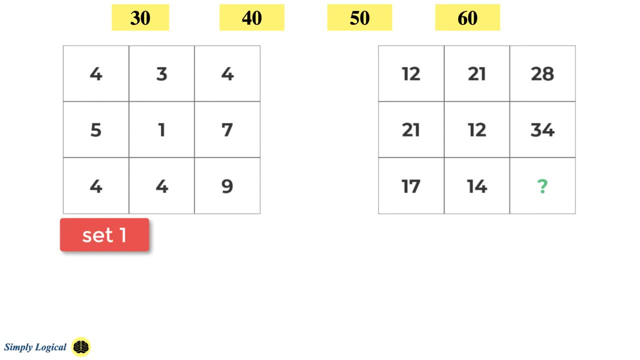 First analyze the numbers in the first set. The trick is add the numbers in each row and check whether it makes sense. Suppose, if it is not making sense, then the second step would be: add numbers in the column. But for now let's add all the numbers in the row and see if we can deduce some kind of relation between the numbers. 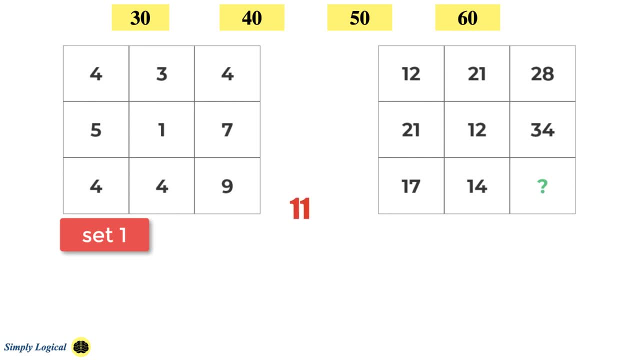 In set 1,, sum of all the numbers in first row is 4 plus 3 plus 4, which is equal to 11.. And sum of all the numbers in second row is 5 plus 1 plus 7 equals 13.. 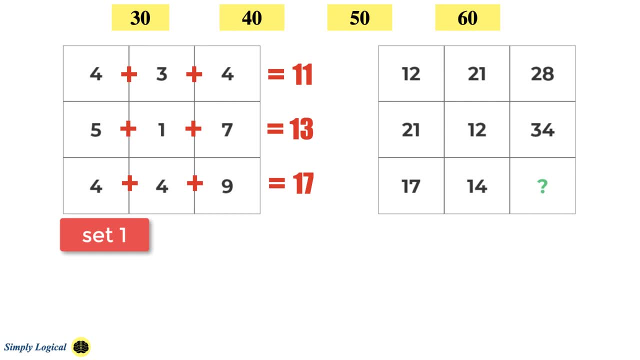 And sum of all the numbers in third row is 4 plus 4 plus 9, which is equal to 17.. So is there any relationship between these numbers? Yes, there is an interesting relation here. That is, the sum of all the digits in the row is a prime number. 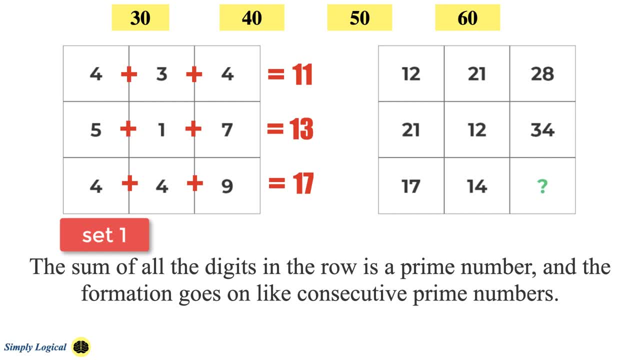 And the formation goes on like consecutive prime numbers. Hope you know what are prime numbers. The prime numbers are those numbers which are divisible by 1 and by itself. For example, 5 is a prime number Because 5 is divisible only by 1 and by itself that is 5.. 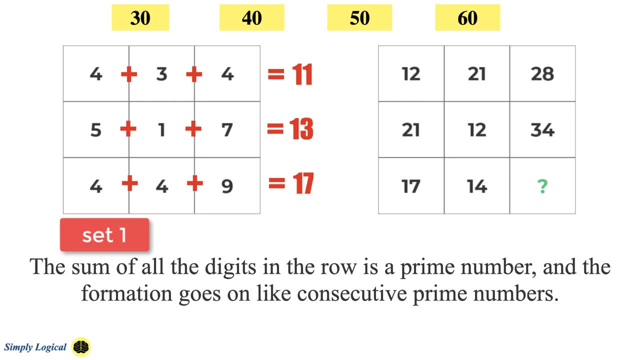 So here, 11,, 13 and 17 are nothing but the consecutive prime numbers. So let us apply the same logic to find the missing number in the second set. In second set, sum of all the numbers in first row is 12 plus 21 plus 28, which is equal to 61.. 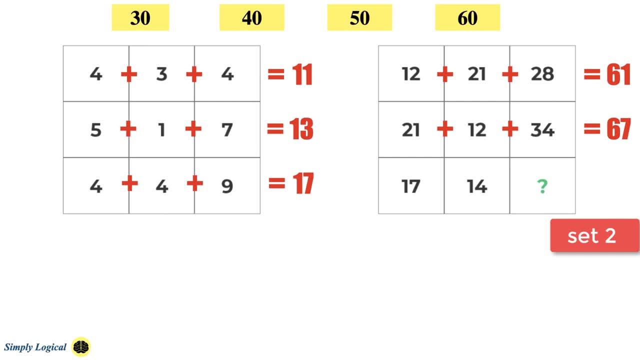 And sum of all numbers in second row is 21 plus 12 plus 34, which is equal to 16.. So sum of all numbers in second set is equal to 67.. So now 61 and 67 are consecutive prime numbers.